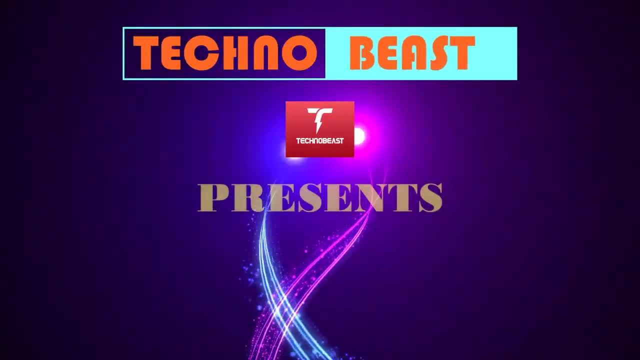 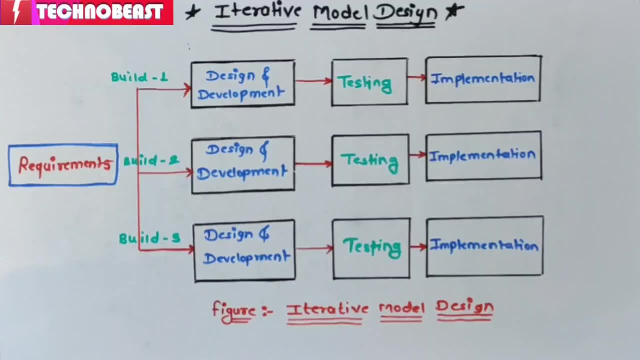 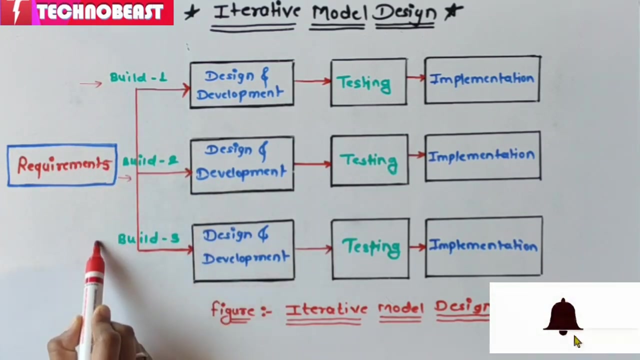 We are going to see the iterative model design. So this is the diagram in which you see there are three builds, that is, build 1, build 2 and build 3.. So this diagram represents that. here is all over the requirements we are collecting in this requirement phase. But as we are going, 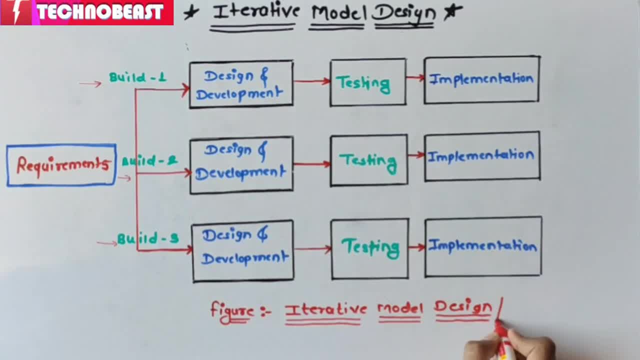 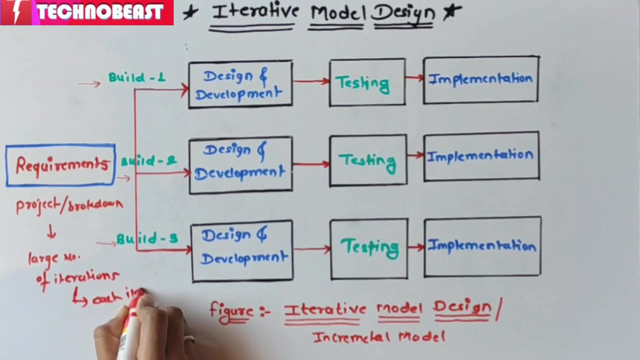 to see that iterative model. we also called it as a incremental model. So we are going to see that outcome, So we are going to see that effect, ok, Ok. So what I am going to say is: here is all project requirements we are gathering here. After that we will broken down into the large number of iterations and in each iteration we get a final product, or we can say that, final software. 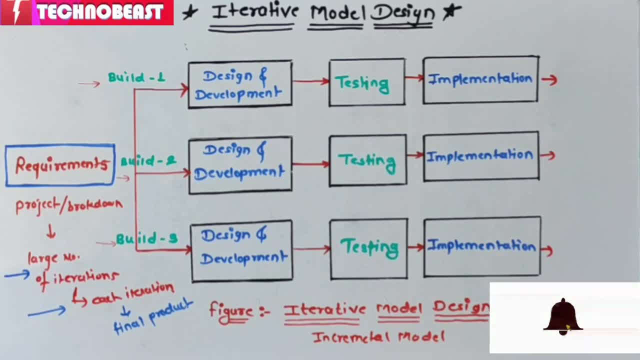 Okay, so in this we are making build 1, build 2, build 3 means in first we will design and develop something, then testing that develop project and then implementing, and after we get the final output right. So in each iteration we are making one product. 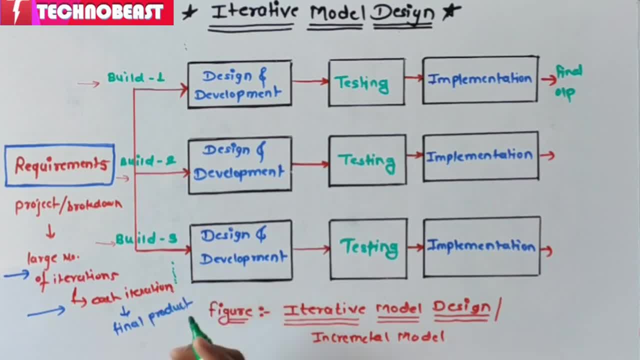 So there are number of build we are making, we can making in this iterative model design. we are also going to say that it is a combination of incremental model. so with the help of this requirement, we are making a small, small portion in each way. again, in second way, we are designing and development, then testing that develop. 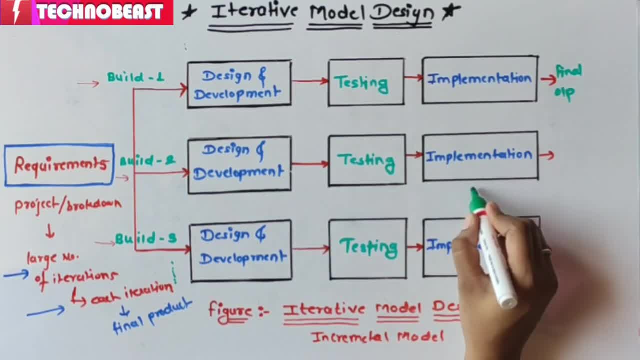 software, then implement it. implement means here we are doing a coding part in implementation phase, right. so after implementing that we are finally deployed, the final output or software. again we are making a build 3, then design and development, testing and implementation. there are n number of built we can make and 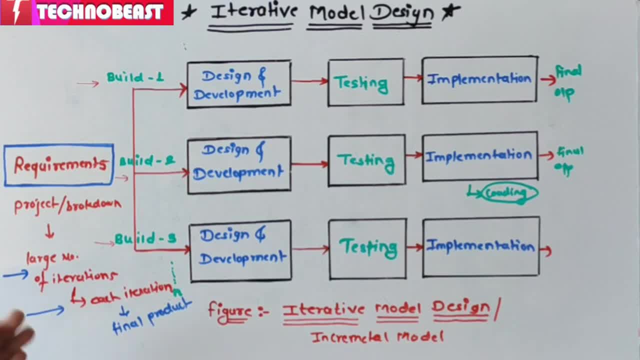 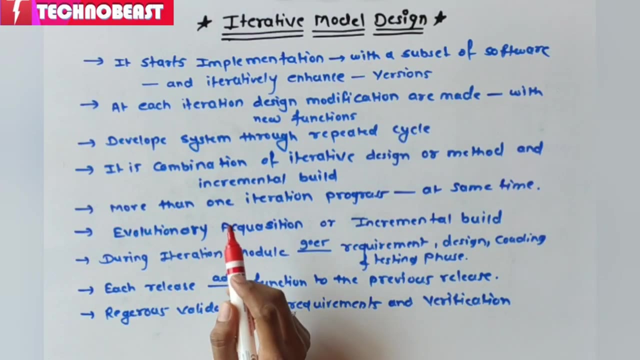 final product will be design. okay, so we are doing until the final product is not get ready. so this is the design of iterative model. that means incremental model. we are already seeing the design of this iterative model. now we will see in details about the build and about the process of this iterative model design. okay, so iterative model. 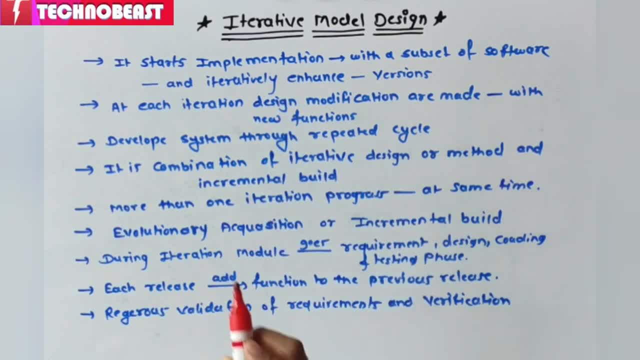 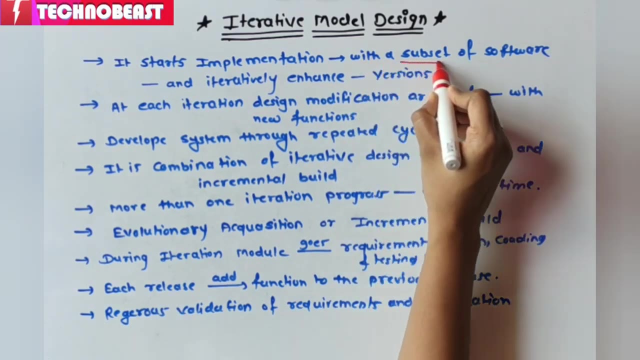 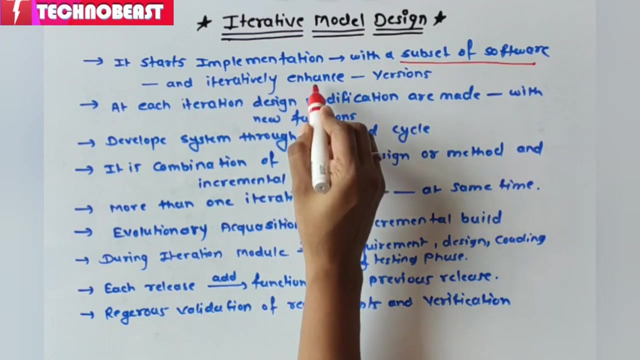 process is start with a simple implementation of a subset of software requirement and iteratively enhance the evaluating version until the full system is implemented. means it is starting with the implementation of subset of the software. okay, subset means small part of the software requirements and iteratively enhance the version. iteratively enhance the versions until 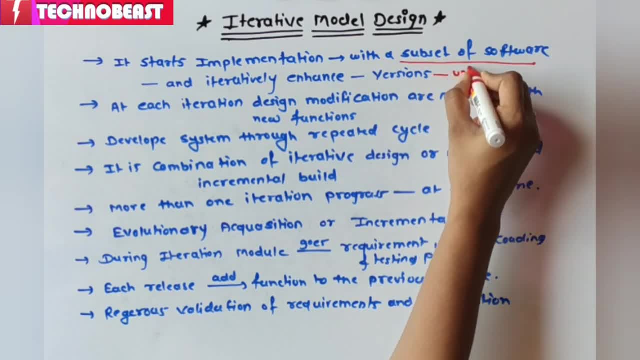 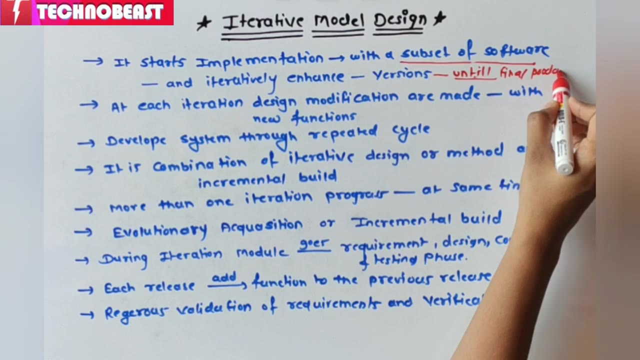 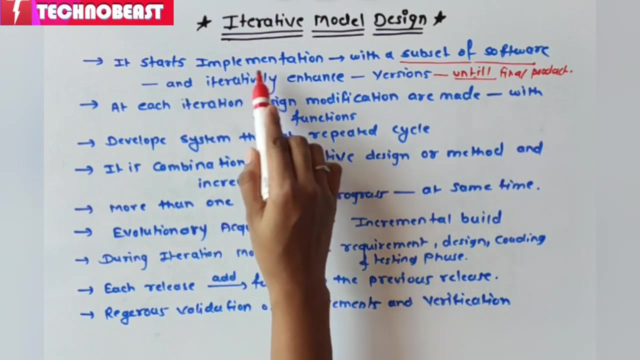 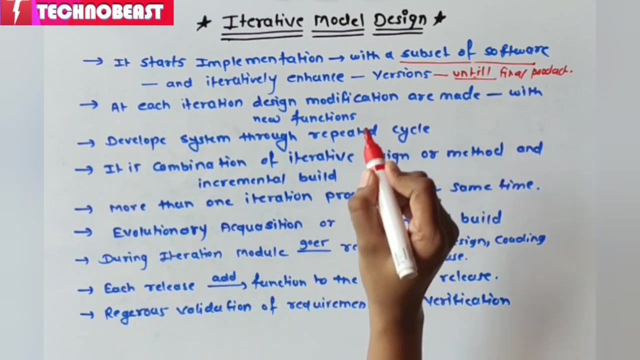 the full system is. implement means this process is continuously in running, sorry, continuously in running until it get a final product. it will get a final product. up till that it will take a subset of software requirement and each iteratively enhance the versions. okay, at each iteration design modification are made, a new functional abilities or capabilities. we can say that. are added means in each of the iteration the design modifications are made with. we can say that new functionalities, right, so these functionalities get added in each iterations. in iterative model the idea behind the method is to develop system through repeated cycle means in which we are doing the system, making idea or developing system through this repeated cycle and smaller portion. at a time. incremental build means smaller portion at a time. right means a big project. we are broken down into smaller parts and making a large number of iterations in this incremental build and we'll using that build for the repeated cycle. okay, so we can say that here is increment, iterative and incremental development. 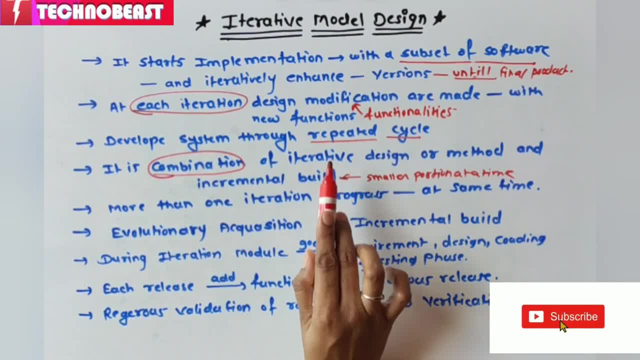 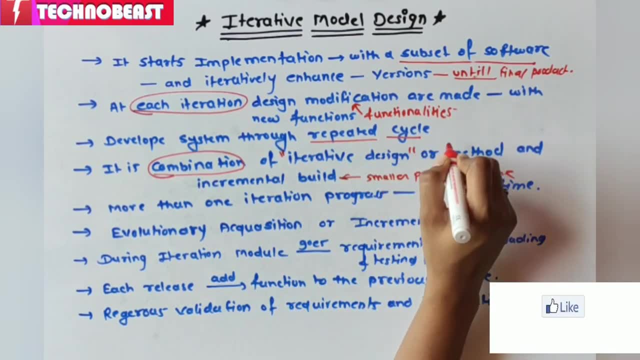 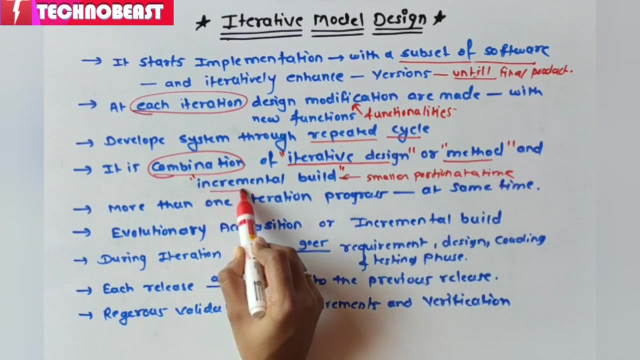 is the combination of iterative design, iterative method and incremental build means this is iterative design, iterative method, and we can say that incremental build- okay. so iterative and incremental is the combination of these three builds right: iterative design, methods and incremental build- okay. so during software development, more than one iteration is. 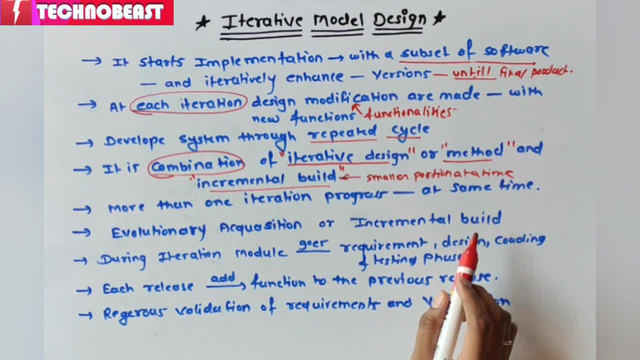 progress at the same time means we can say that whenever the development of software is uh processing, more than one iteration of the software development cycle may be processed at the same time. means if there is a one iteration will be in progress. so there are so many iterations will be in. 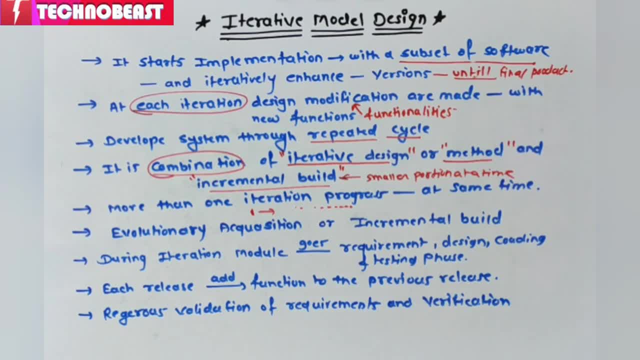 work in progress means there are another versions, will still working on that okay. means we can say that this process can be described as a evaluationary acquisition, right. or we can say that it is a incremental B approach. what we can say that incremental B approach: okay, in this incremental model, the whole requirement. 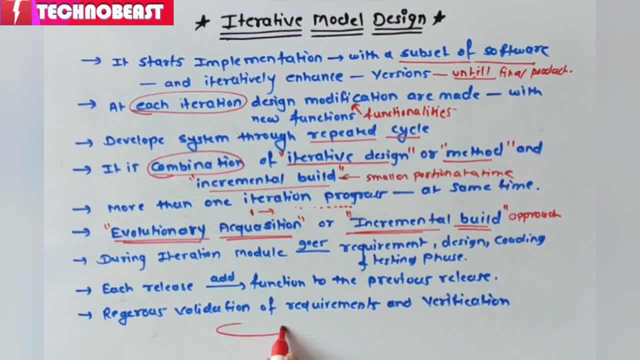 is divided into various. bill means your whole project is divided into the smaller parts of the version of the software. you can say that small build they are making okay. during each iteration the development module goes through the requirement: design coding. we can say that implementation and testing phases okay. so each subsequent release of the module. 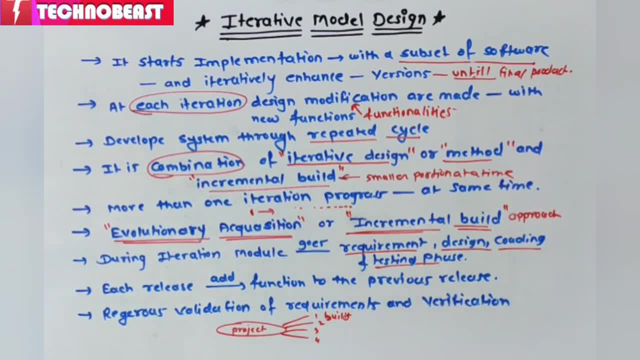 add function to the previous release means whatever the comes in market, then they will be adding a new function to the previous one. means each release add new functionality. right, the process continue till until complete system is ready, as per the requirement. and this process is continue up till a final system get ready.